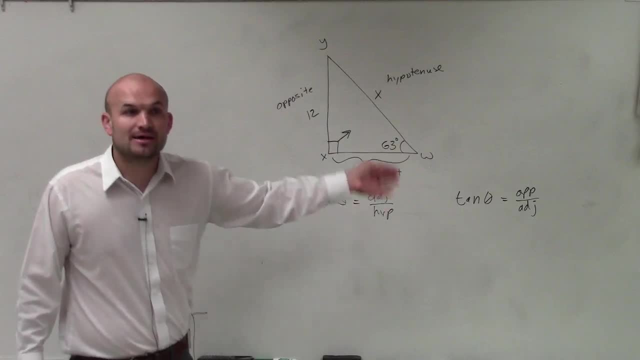 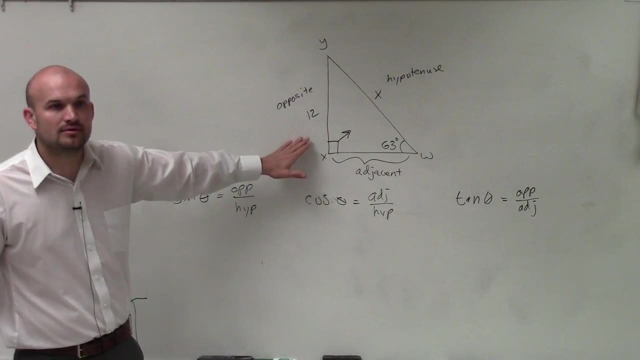 one as a number and one as a variable. And so, by looking at those two, as one is a variable, one is a variable, Dennis, what are we provided? What is our 12?? Our 12 is what? What side is the 12? Adjacent? it's the opposite, And the x is. 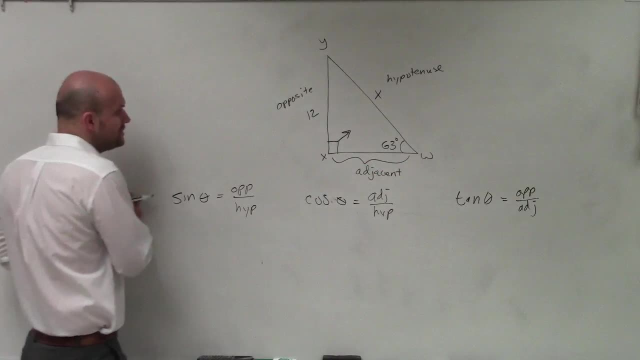 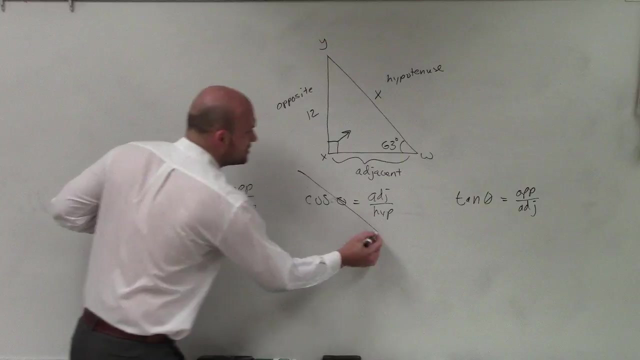 We don't have any adjacent right. So, Dennis, what is the only trigonometric function that deals with opposite and hypotenuse The sine? So, therefore, we're not going to do cosine, We're not going to do tangent, We now need to solve using the sine function. 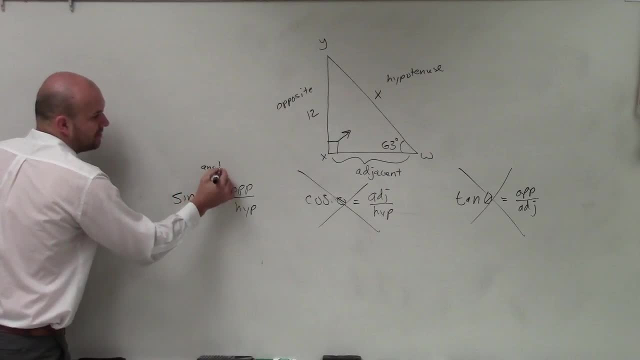 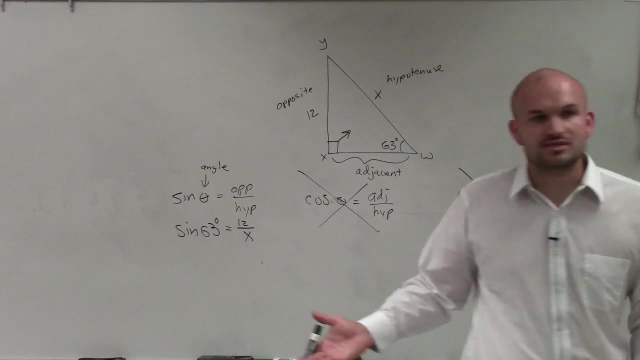 So remember, theta represents our angle. So now I do: sine of 63 degrees- because the trigonometric functions are functions of an angle- is equal to the ratio of 12 over x. Now, this one was a little bit more difficult than what we went over, but, guys, now it's just basic algebra. So now we need: 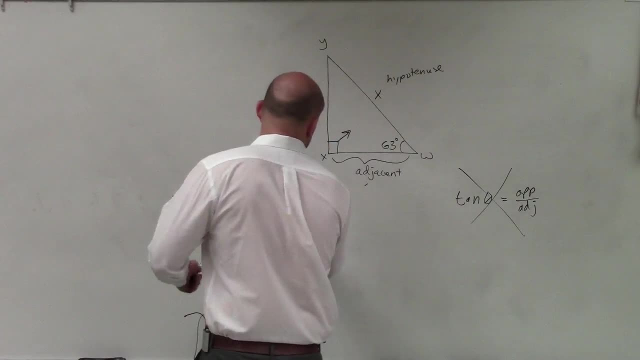 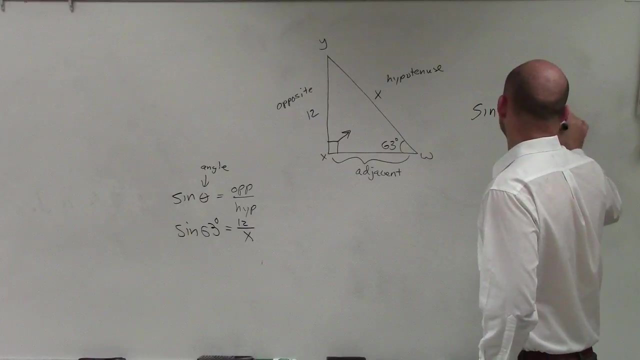 to solve for this, And I'll actually do it over here. And I'll actually do it over here to show a little bit more work. So sine of 63 degrees equals 12 over x. When we're trying to solve for x, we have to get the x off the denominator. So what I'll do is I'll 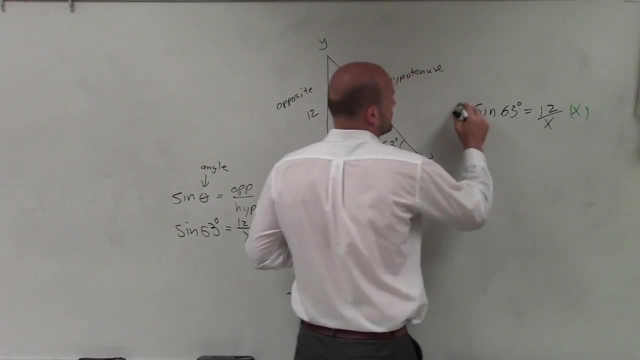 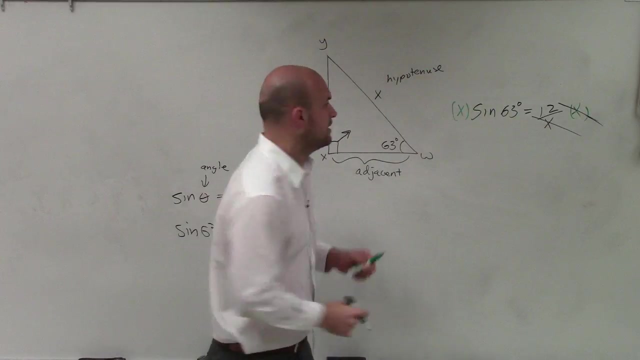 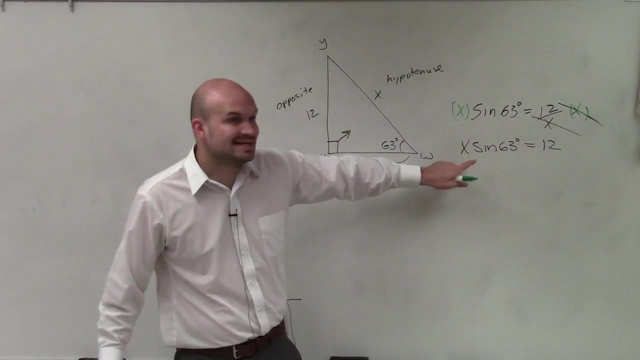 multiply by x on both sides. I multiply x on both sides. These now divide to 1, and I'm left with x times the sine of 63 degrees equals 12.. Now again I need to solve for x, correct? 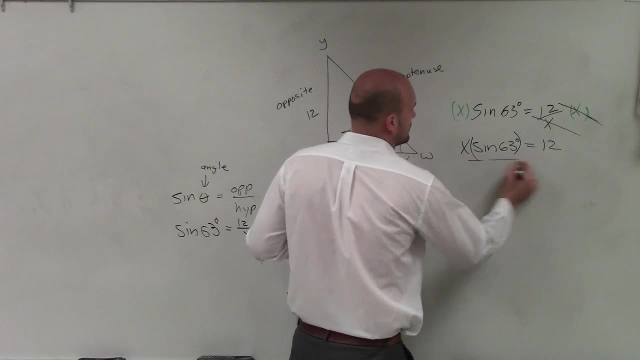 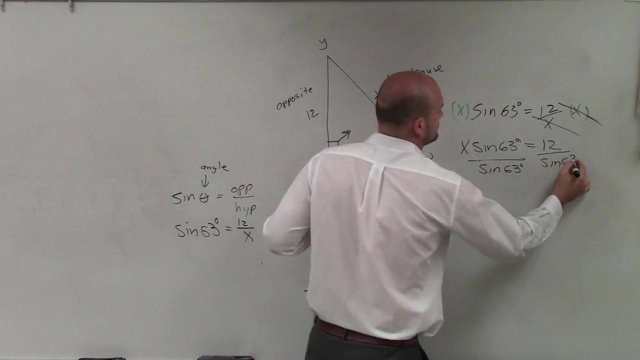 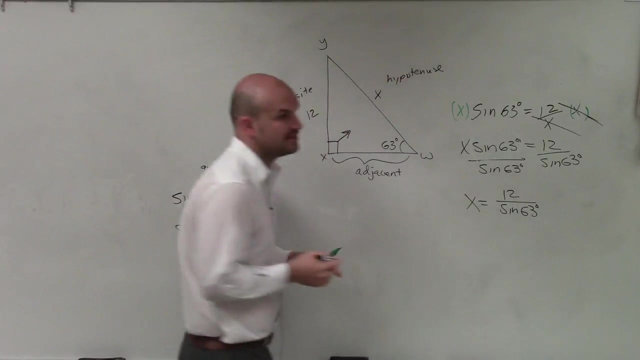 So what I'm going to do is I'm going to divide by sine of 63 degrees. I don't know why I did that. Therefore, x equals 12 divided by the sine of 63 degrees. Now, we're not done yet. 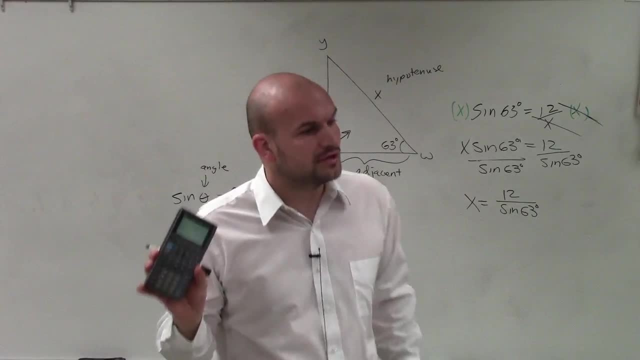 We still need to go ahead and plug this in our calculator. So we want to make sure our calculator is in degree mode, And if you don't know if it is, I can show you, or at least help you, how to put it into mode. 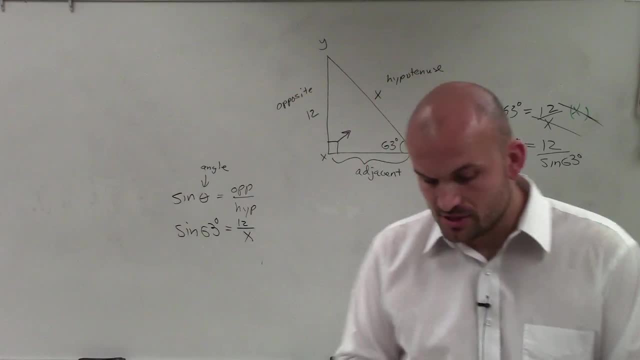 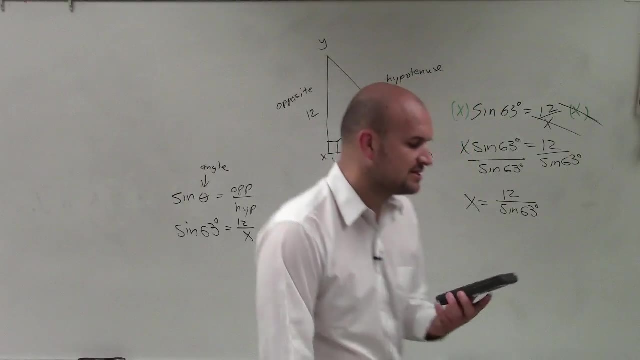 It should automatically be in degree mode, but it could also be in radian mode. So I'm just going to take 12 divided by the sine of 63. And my answer is 13.4.. So therefore, x equals 13.47.. 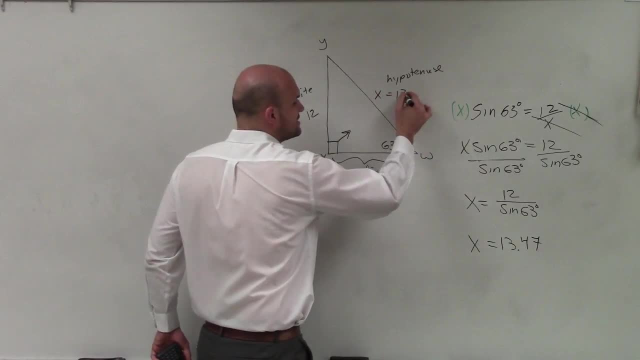 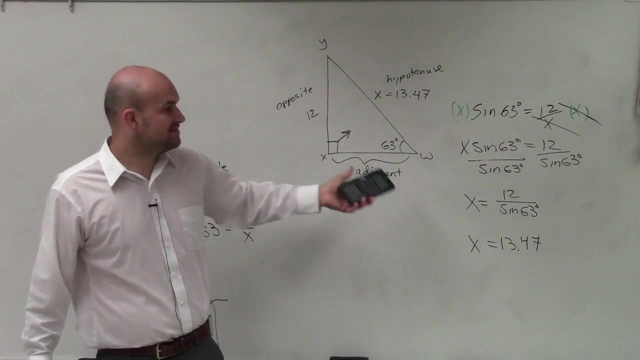 I'm going to round to the hundreds Now. ladies and gentlemen, does that make sense in this triangle? Does that sound like a real thing? Is that a reasonable number for my hypotenuse to be? Sometimes, if you get a radian and it's like 2,, 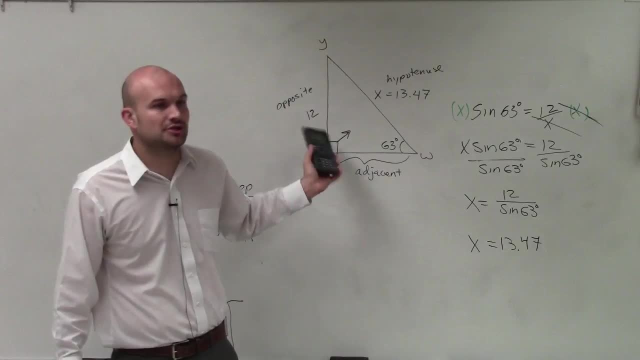 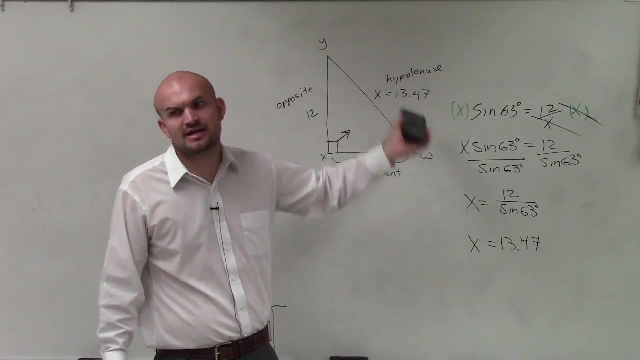 well, obviously you know the hypotenuse cannot be 2 if one sine length is 12, right. So then you know you did something wrong. Or if this hypotenuse was like 856, okay, something's wrong, because that should not be that large. All right, All right. 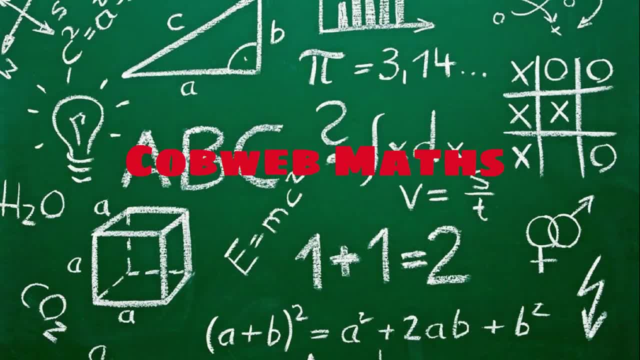 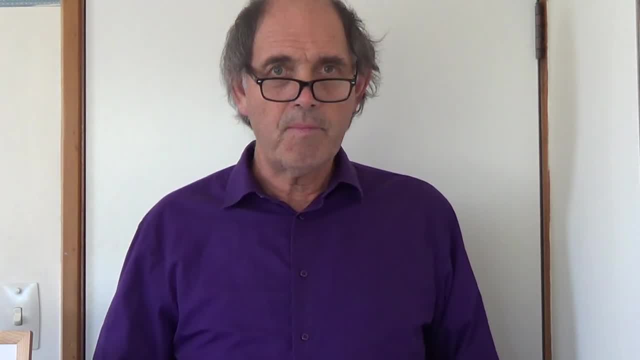 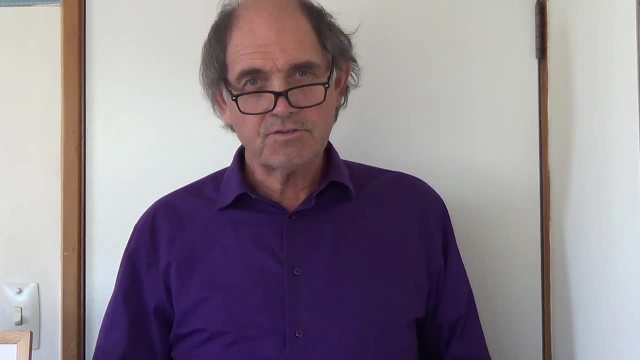 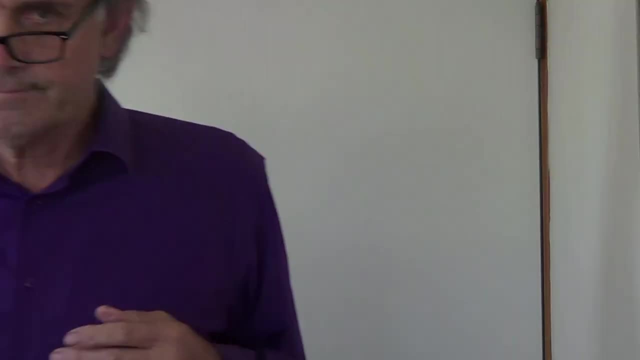 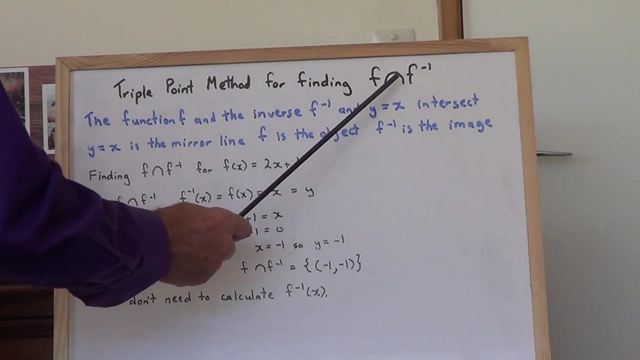 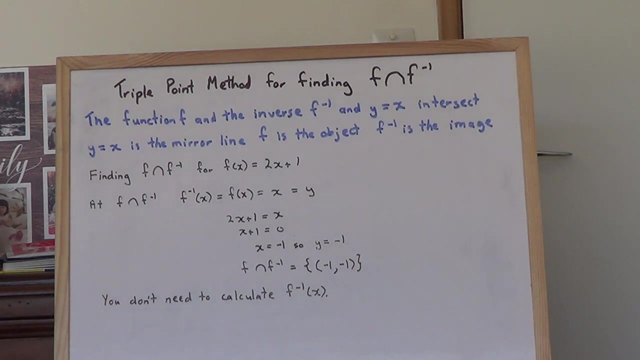 I'm Craig Grant and this is Cobweb Maths. Taking a wider view can often lead to easier ways of doing things. That's exactly what I do in this video. This is the triple point method for finding a function intersected with its inverse function, and that's going to be actually a point Now. this 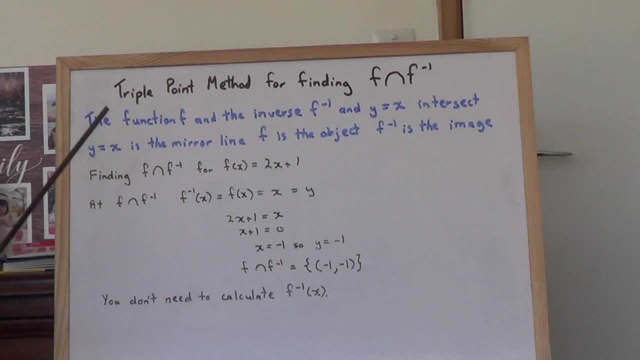 is the basis of the triple point method. You've got a function, the inverse of the function, and the line y equals x and these three things intersect and the intersection gives you this, So it's actually a triple point intersection. y equals x is the mirror line. 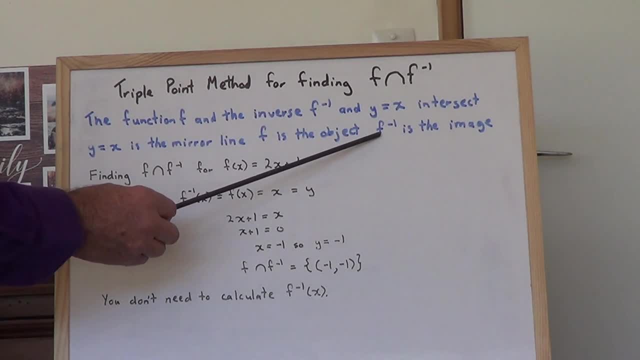 f is the object and the inverse of f is the image. Now we're going to do a question. We're going to find f intersection f to the minus 1 for this function here, 2x plus 1.. So what you need to 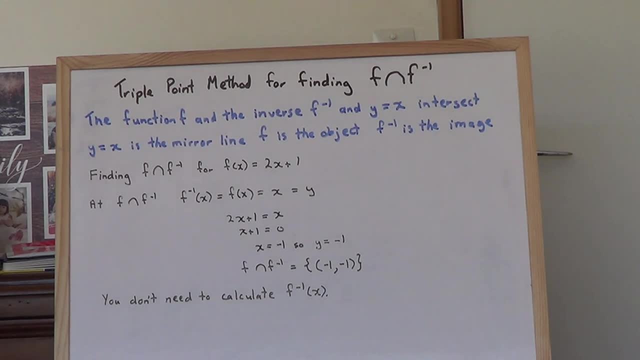 do is explain to your marker if you're doing an external exam, what you're actually doing. So you say at f intersection, f to the minus 1, f to the minus 1 of x is equal to fx is equal to x is equal to x, And then basically you just focus on these two: 2x plus 1 equals x. Take x from both.